ideas, you will be able to make a good use of the recycling business idea. Secondly, after the selection of the recycling business idea, have a thorough knowledge of the recycling business idea. By taking up any of the recycling business ideas, you are protecting the 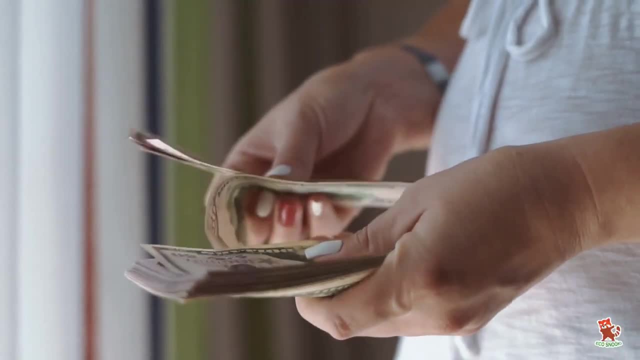 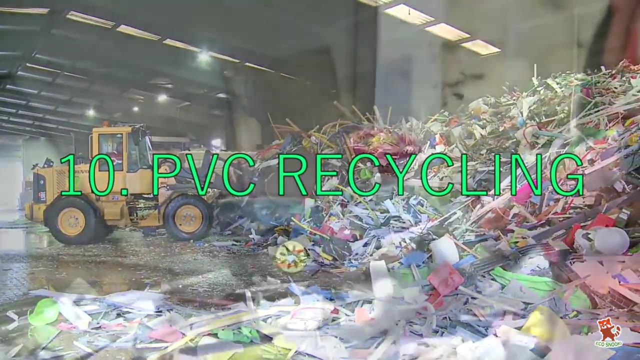 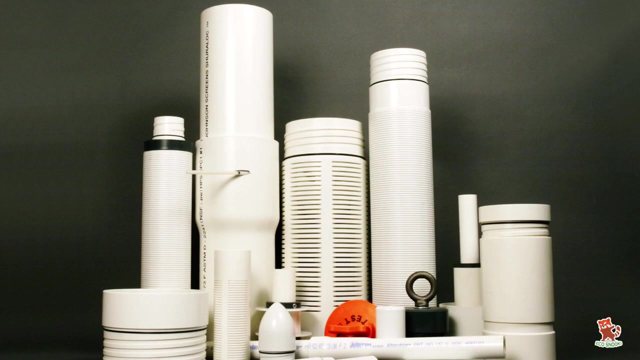 environment at one hand, and earning profits on the other. Here we have 10 most profitable recycle business ideas. Number tenth is PVC recycling. PVC, or polyvinyl chloride, is used mainly in the manufacturing of pipes, shades, tanks, etc. You can take the rejected PVC, treat them and 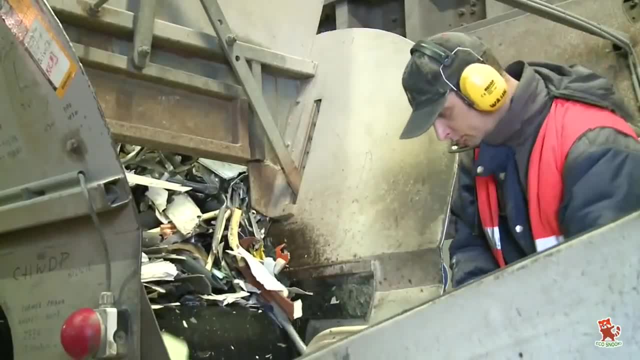 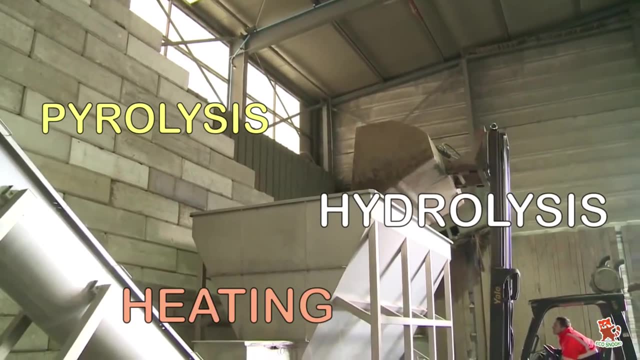 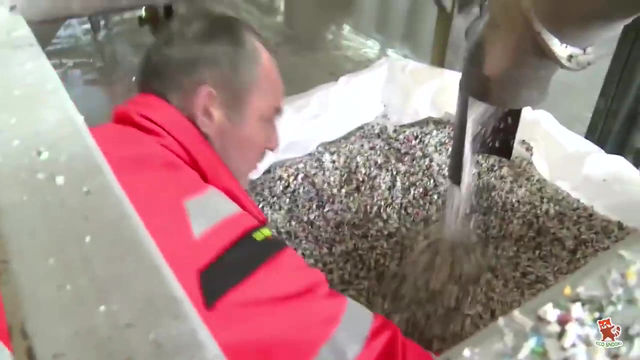 manufacture other goods of PVC. This is a common and useful recycling business idea. Chemical process is, such as pyrolysis, hydrolysis and heating are used to convert the waste into its chemical components. The resulting products: sodium chloride, calcium chloride, hydrocarbon products. 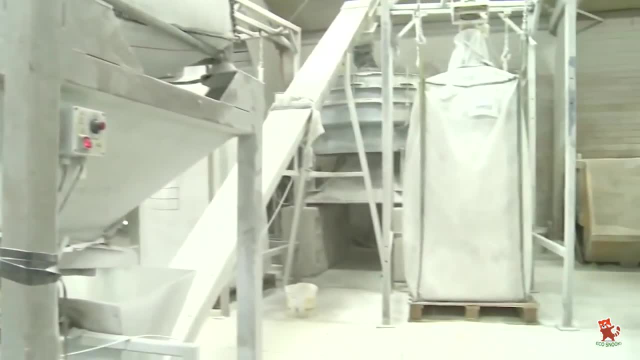 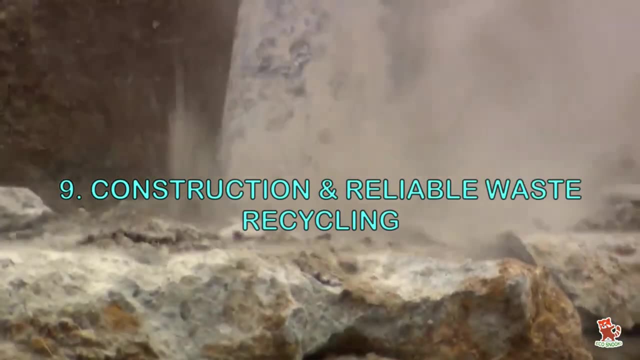 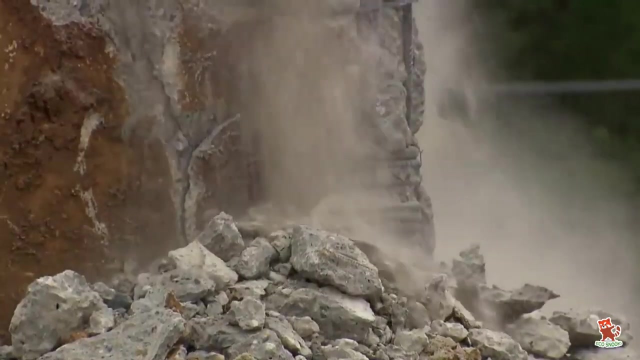 and heavy metals, to name a few, are used to produce new PVC as feed for other manufacturing processes or as fuel for energy recovery. Number ninth is construction and reliable waste recycling. Generally, solid wastes are non-biodegradable and untreatable. You can collect these. 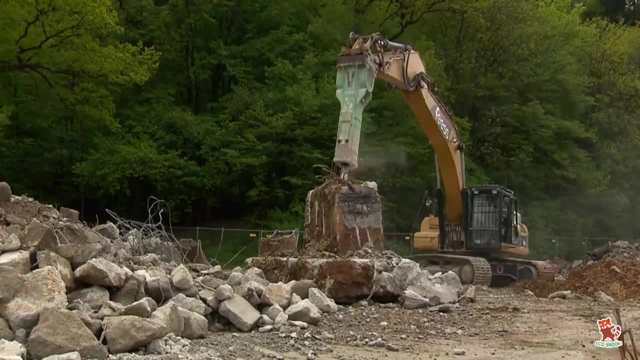 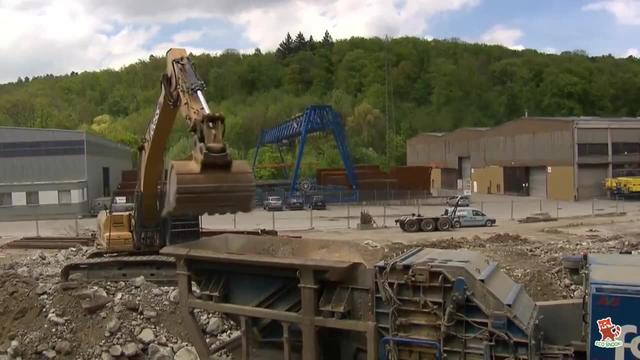 solid scraps from the construction sites and manufacture it into bricks. After doing treatment of these wastes, then, after compressing, the new shape can be given, which is stronger, having a long life cycle. These bricks can be sold to the nearest construction houses in small units. 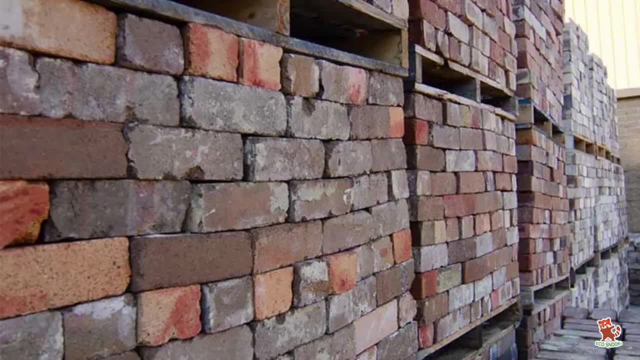 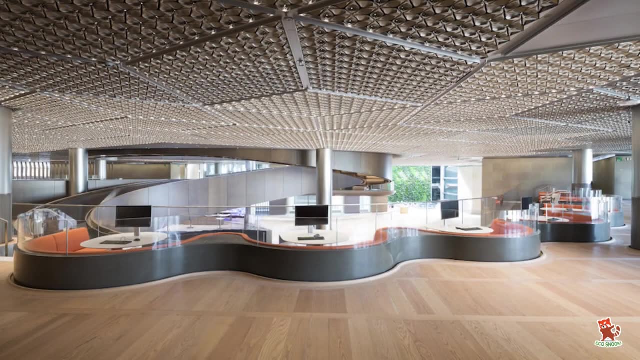 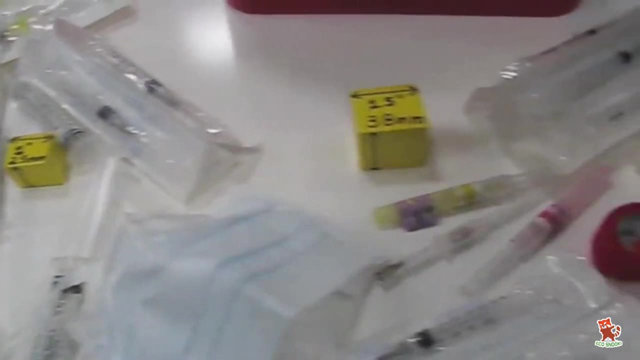 and by signing the contract with builders you can trade in bulk also And also you can use interlock tiles, partition boards, false ceiling materials, etc. on second use after small repairing and painting. Eighth is medical waste recycling business. As you know, medical wastes are in most cases unhealthy and hazardous. 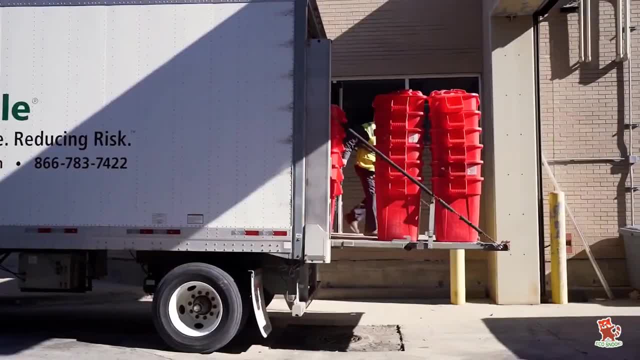 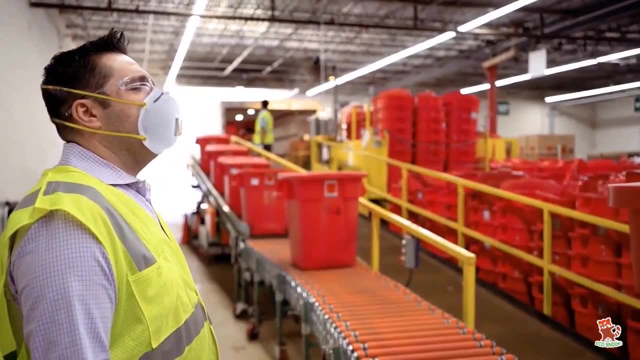 Here you can prove yourself of great help for the hospitals and society, along with making profits for yourself. A large portion of medical wastes like syringe and needles can be recycled: Autoclaving gas, sterilization, chemical disinfection, microvave irradiation. 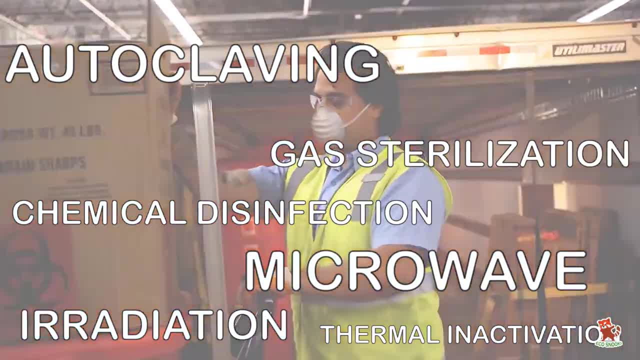 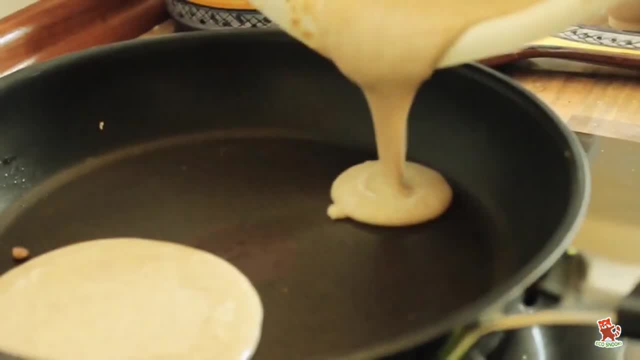 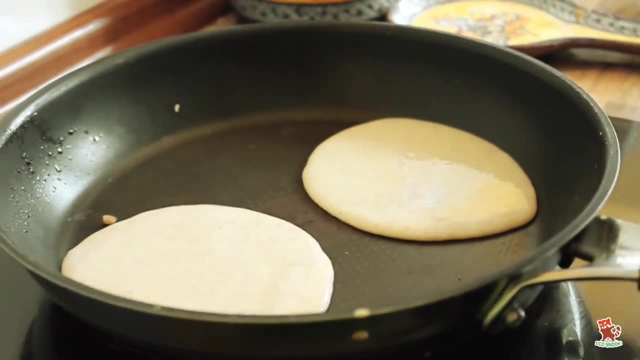 thermal inactivation, etc. are the main methods used to recycle medical waste Utensils. recycle business on number 7.. It's possible to be wasteful in the kitchen without even realizing it. All of the activities that are routinely carried out in the kitchen: cooking, cleaning and eating. 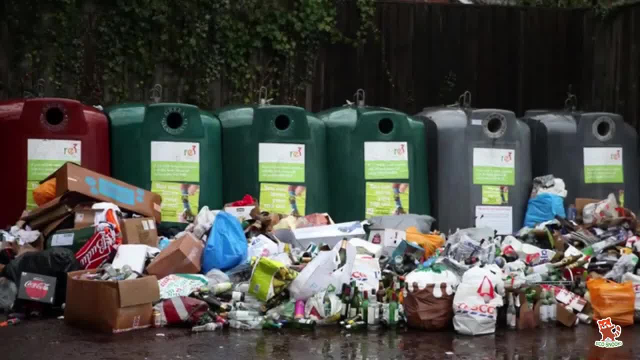 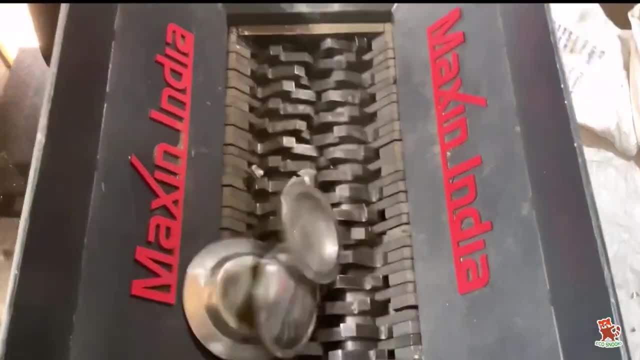 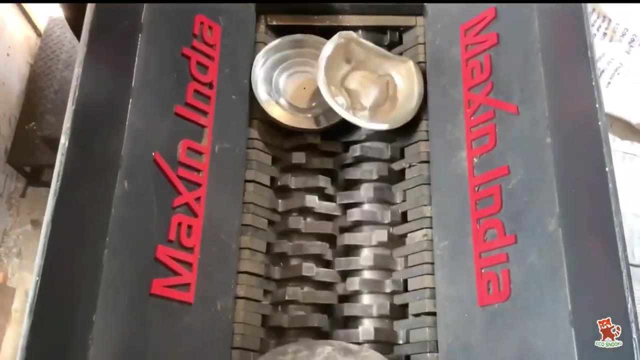 produce significant levels of waste. We often reject or throw away our old utensils, But these utensils can be the source of your recycling business idea. Most of the utensils are made of steel, copper or iron. In your recycling unit you can process them and make new utensils. 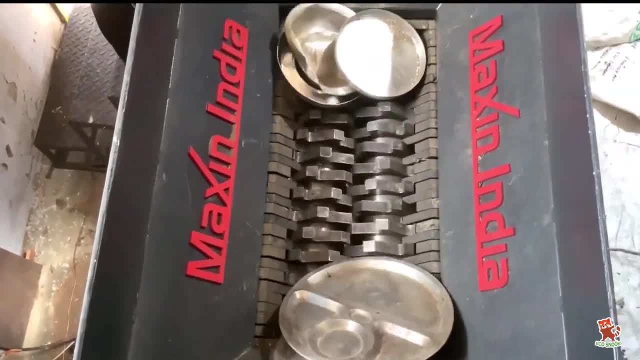 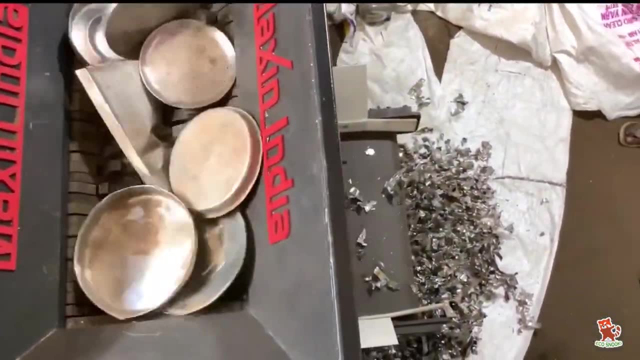 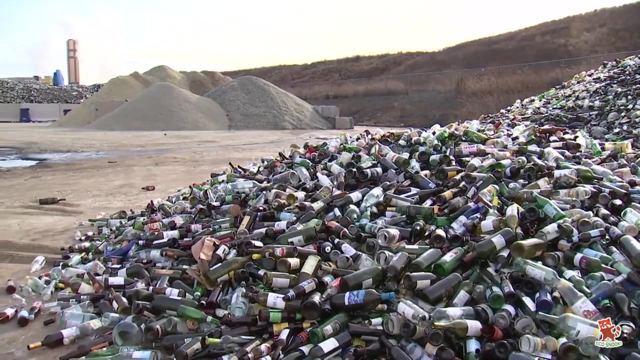 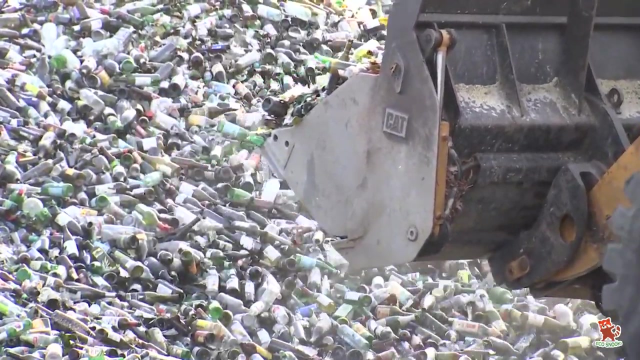 You can sell them to other business persons Or you can sell them directly to earn profits. Number 6 is glass recycling. The commercial glass recycling statistics reveal that there is room for improvement amongst businesses and industry. Within the hospitality industry alone, pubs, restaurants and bars send 200,000 tons of glass to landfill each year. The glass recycling 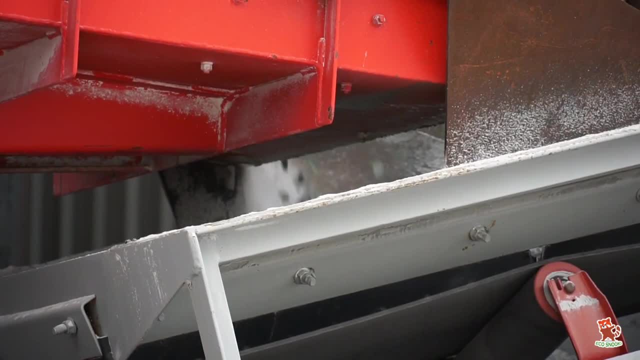 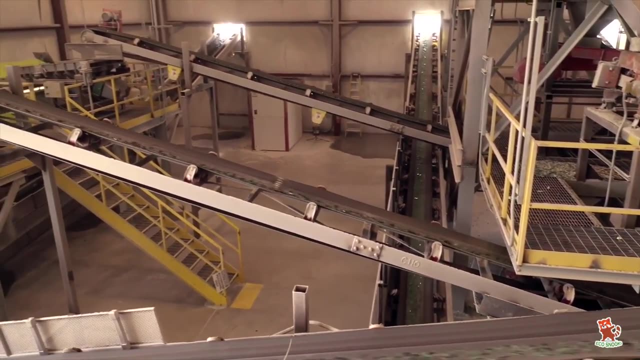 is a relatively easy material to melt down and remake into many different kinds of shapes, From drinking glasses to molded sculptures, to glass fiber. it's a material with innumerable uses in the world today. Once collected, the glass is broken up into smaller pieces. 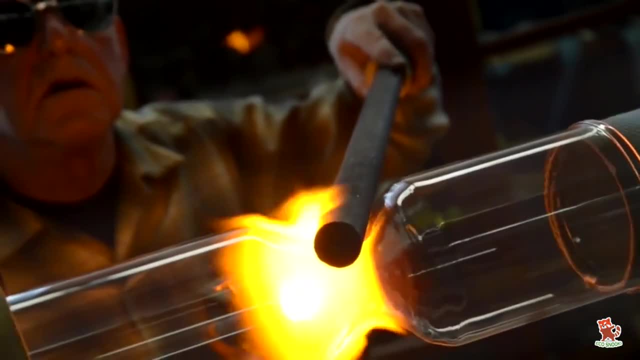 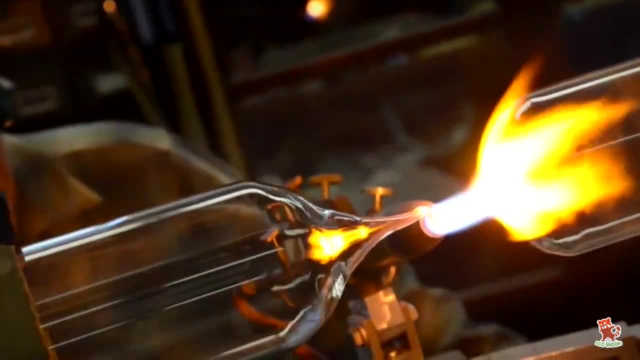 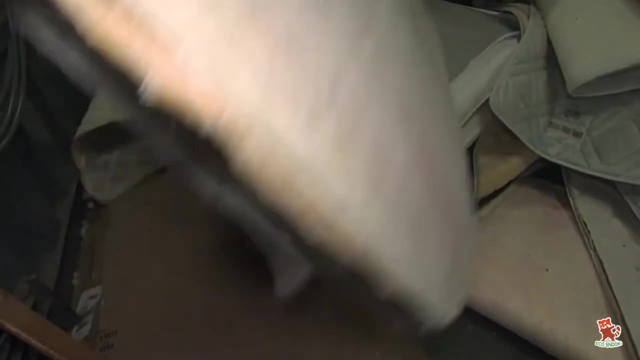 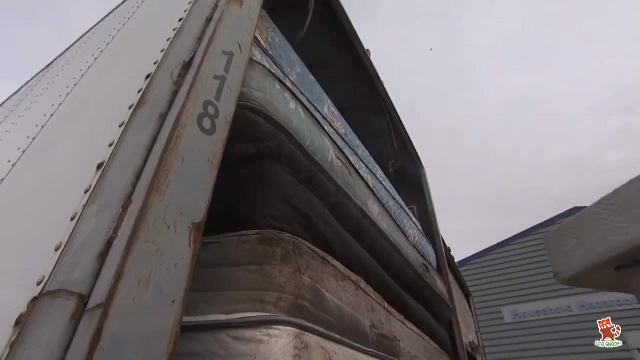 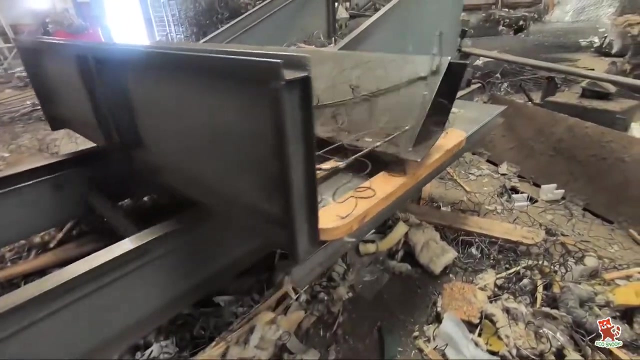 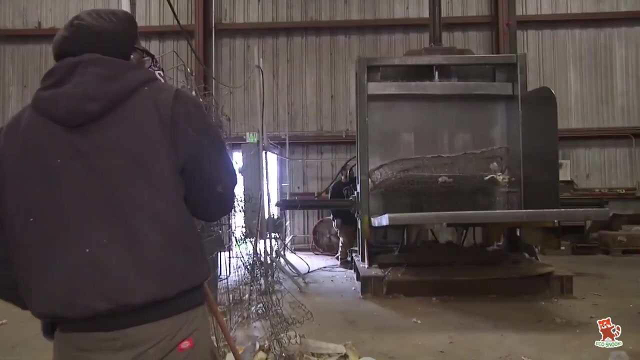 crushed, sorted and cleaned. It can then be mixed with other constituents like sand, then melted and molded into the desired shape. Number 7 is glass recycling. The commercial glass recycling statistics reveal that there are no each other and recycled at a success rate of 95 percent. the mattress plants usually send the 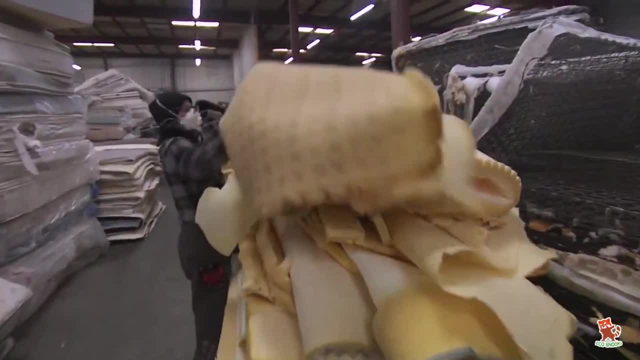 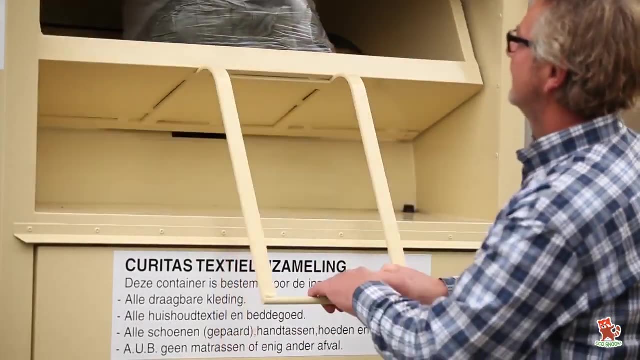 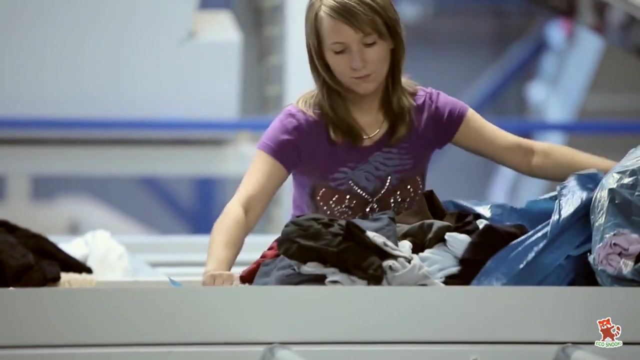 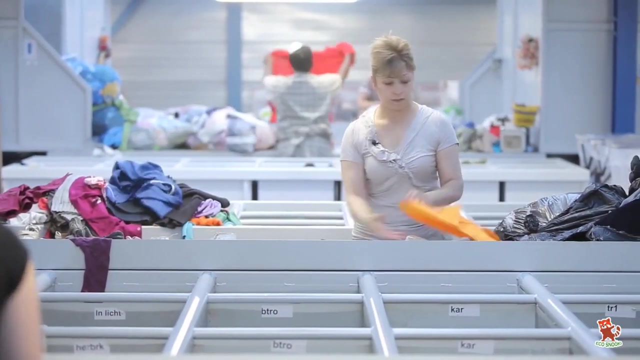 constituent materials to specialized plants that carry out the actual recycling process. textile recycling on number four. textiles like pieces of clothing and parts of sofa sets make up a significant portion of most landfills. used clothing can normally be reused by making small changes on them, while others have to be recycled. during the recycling process, the textiles are: 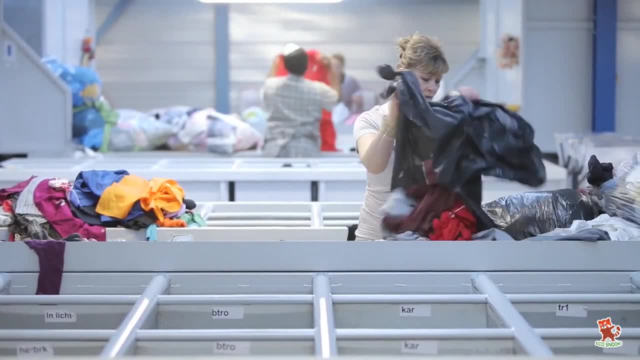 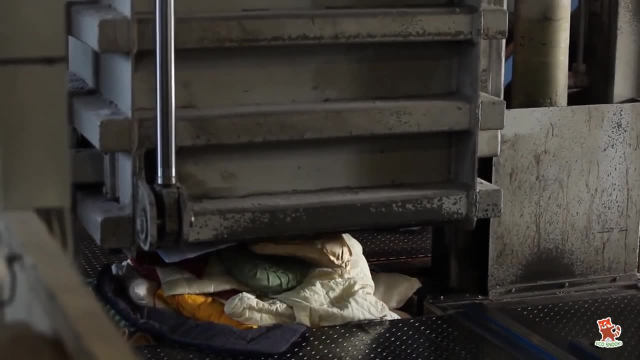 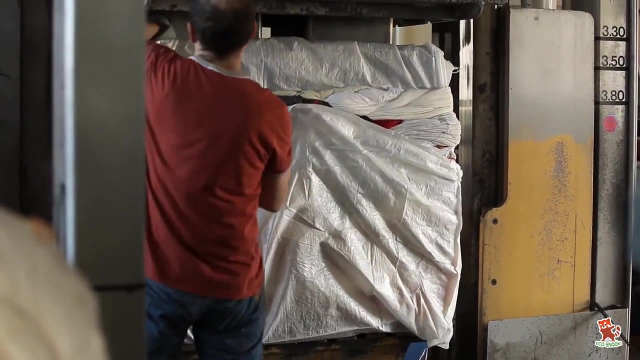 sorted based on the type and processed into different categories depending on the color and type. these can then be reused in the manufacture of new clothes or for reinforcing some types of furniture. for your textile recycling business to be sustainable, you must ensure that have a steady supply of unwanted textiles being collected. as such, you'll need to call upon the 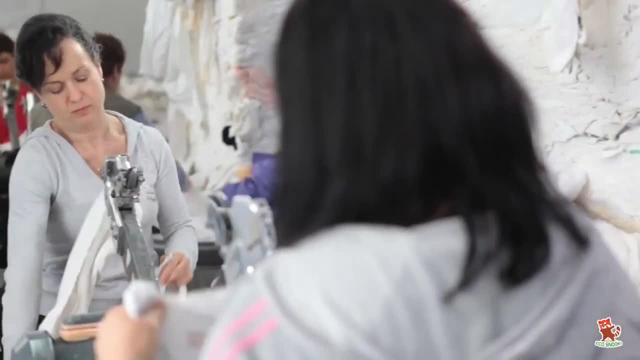 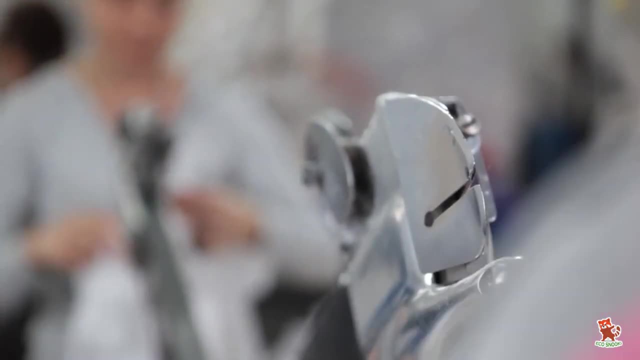 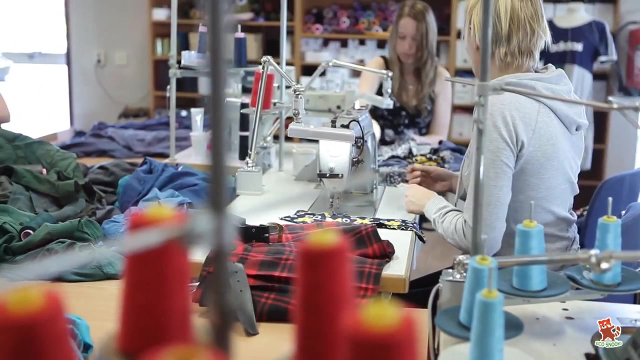 help of your local community, making it as convenient as possible for them to discard unwanted clothing. one way of achieving this is by seeking permission to place textile banks in car parks or along high streets. plus, you'll need to factor into your decision how much it may cost to have any deposited clothing transported back to your business. 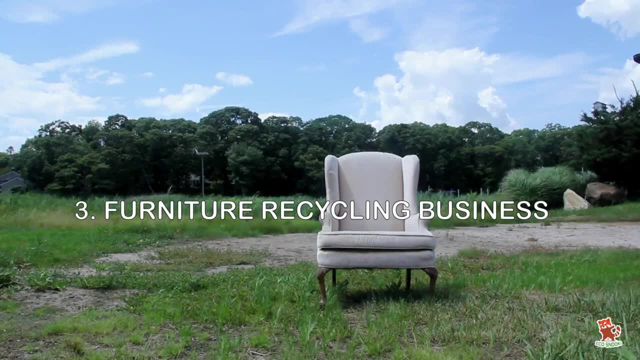 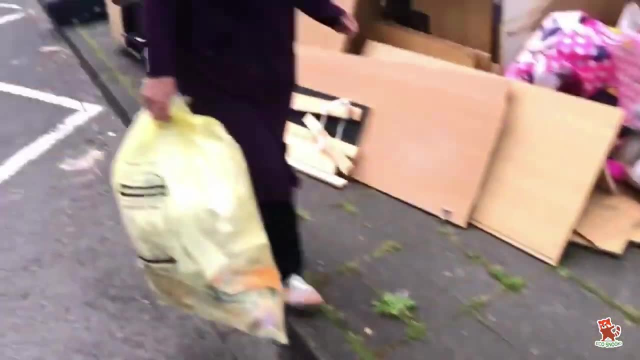 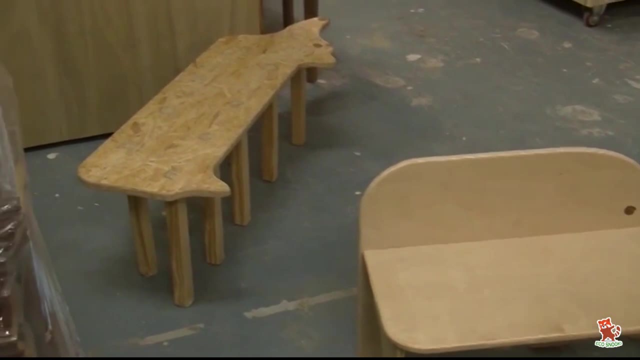 number third is recycling junkyard furniture. recycling junkyard furniture requires a considerably larger amount of creativity and workmanship than others on this list. however, creating usable furniture from discarded pieces is a very profitable venture. lots of people like to buy unique kinds of furniture, based on them being uniquely made, if possible. this can be. 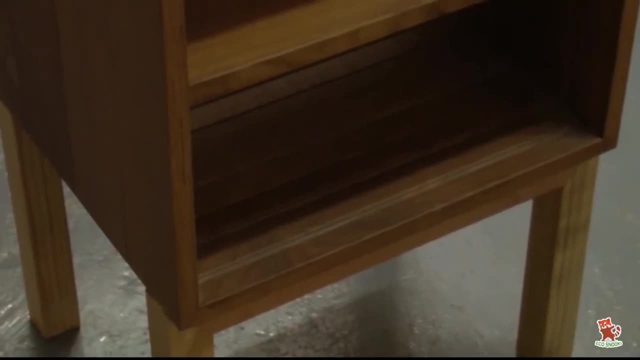 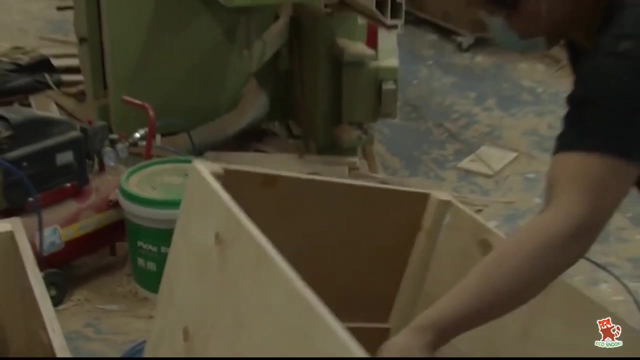 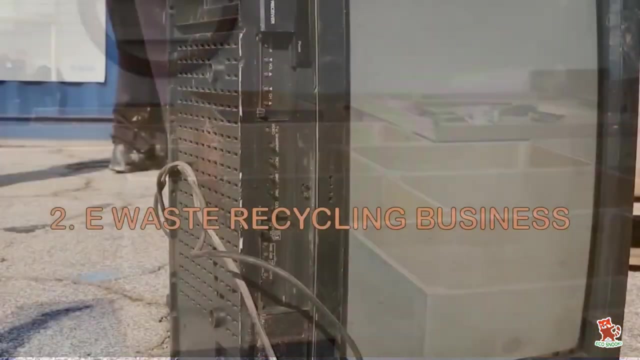 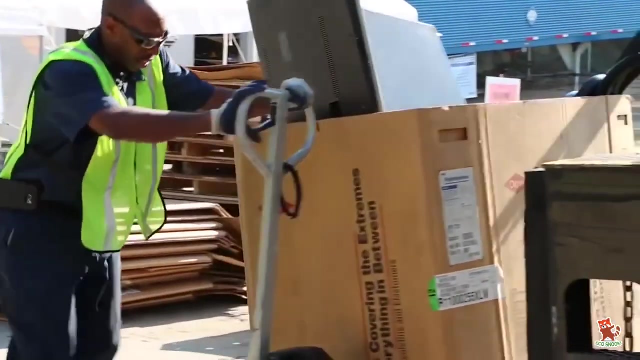 combined with textile recycling. perhaps the most attractive thing about a furniture upcycling business is that you can open it very cheap. for instance, it is very possible to open such a business for two thousand dollars or less. electronic waste recycling. on second position, the waste which contains cadmium, phosphorus, lead. 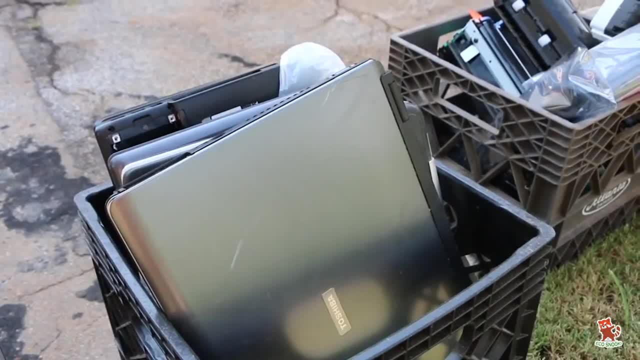 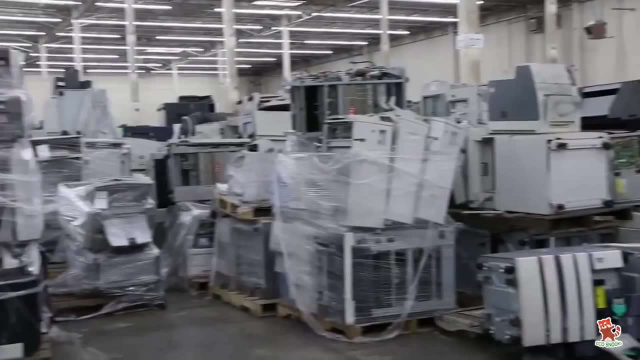 etc. which came out from the electronic waste items is highly valuable and profitable but due to some dangerous metals, you need to take some precautions and must have experts in your team. you have to take the clearance and make your documents ready as per the government norms. it is also considered: 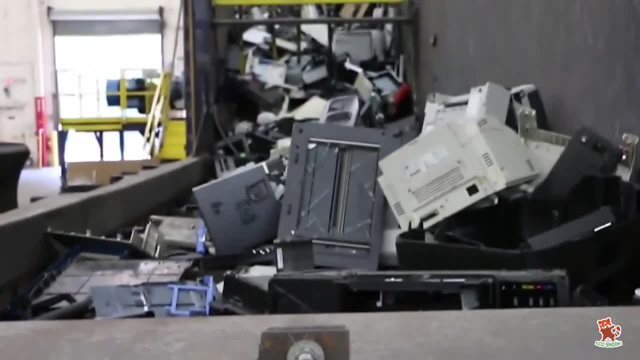 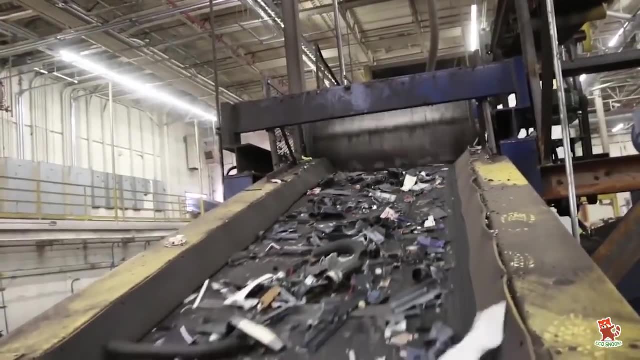 one of the best ways to save money to search the place and find it is the safest way to hire an way to save Mother Earth by being eco-friendly. with the holistic marketing concept, By taking some precautions, you can make a considerable profit with high return on investment. 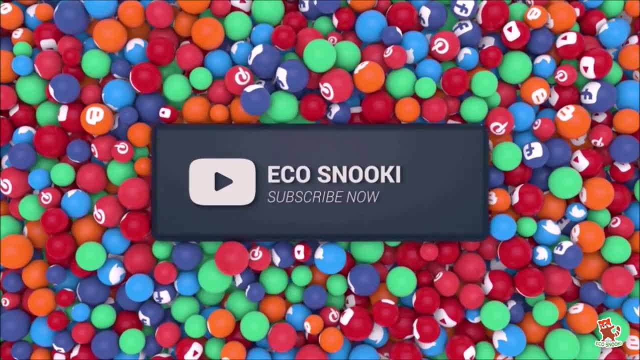 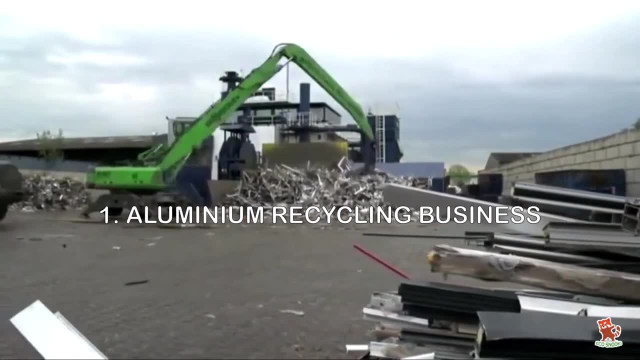 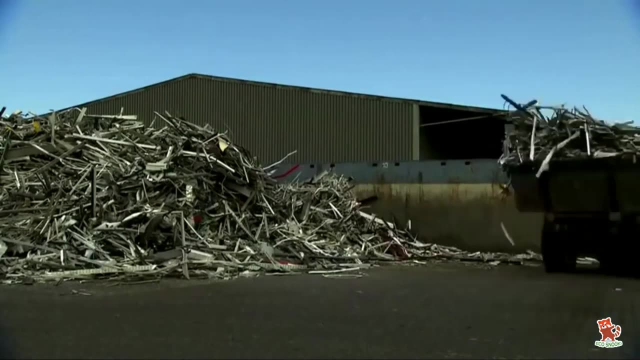 Before moving forward, please subscribe this channel for more interesting videos related to nature, energy and sustainability. From our studies, we found that aluminum recycling is the best recycling business, with minimum wastage of material and best profit, So this comes at first position. 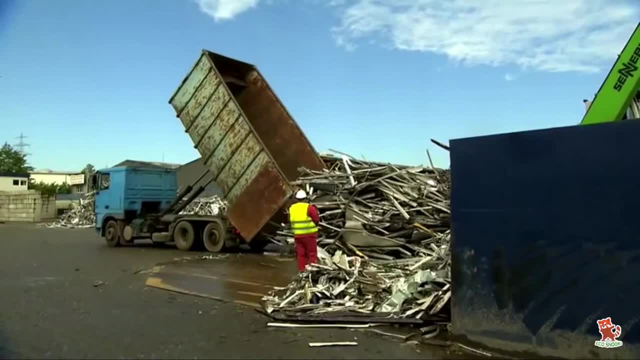 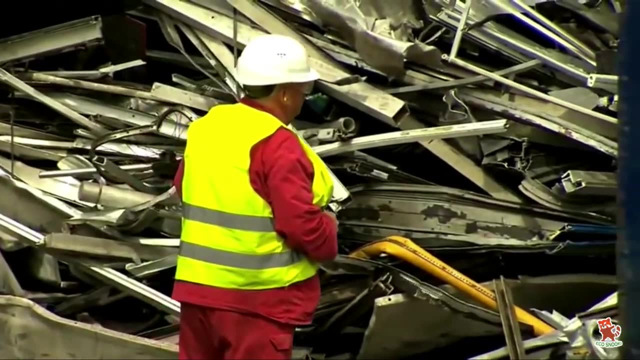 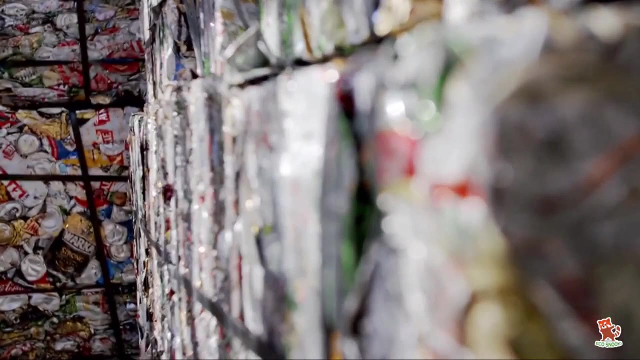 Aluminum is the most recycled metal in the world with the least risk. The usage of aluminum is widespread and almost everybody is using it. If we talk about the most common thrown material, that will be aluminum cans. This is a hassle-free recycling business idea for you on one hand.